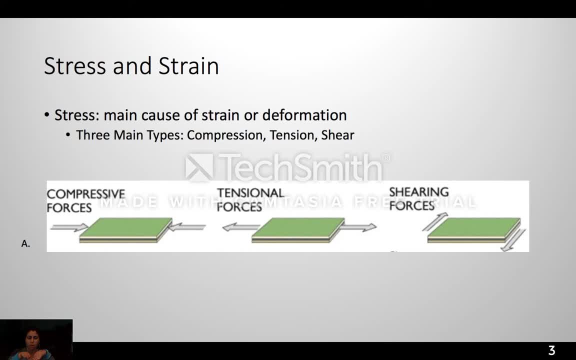 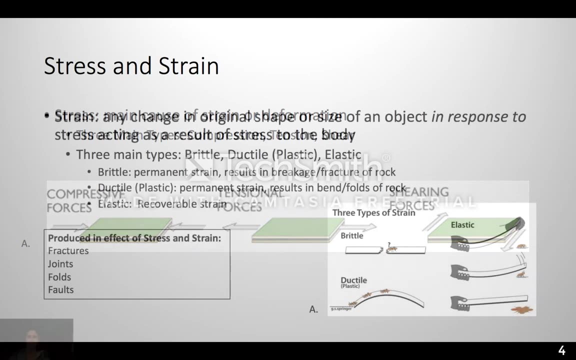 So it goes back and forth, side by side. Faults and folds are the architecture of the earth's crust and are the effect of each of these different types of stresses in different variations. Strain, along with stress, definitely plays a role in the movement and deformation of the plates. 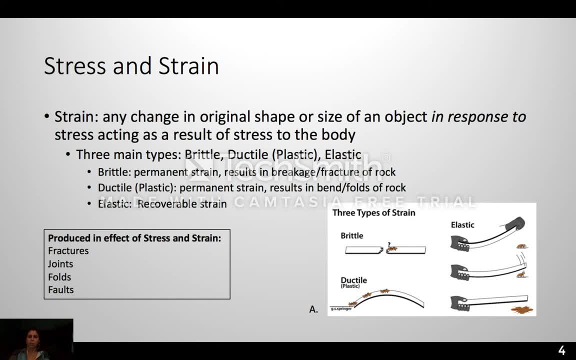 Strain can be defined as any change in the original shape or size of an object in respect to the movement and deformation of the plates. Strain is a response to stress acting as a result of stress to a body, So strain is basically an effect of stress. 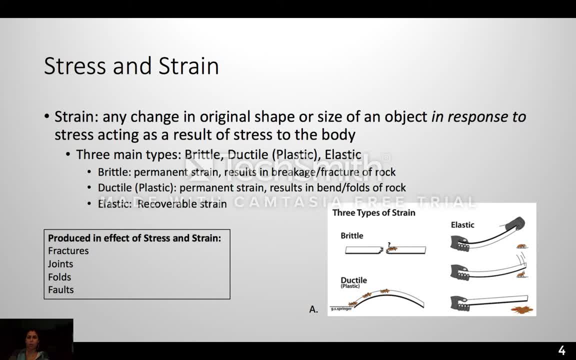 There are three types of strain: Brittle, ductile or plastic, and elastic. Brittle strain can be described as a permanent strain. It typically results in rock breakage or fracture. It cannot be recovered back to the original. Ductile or plastic strain is also a permanent strain. 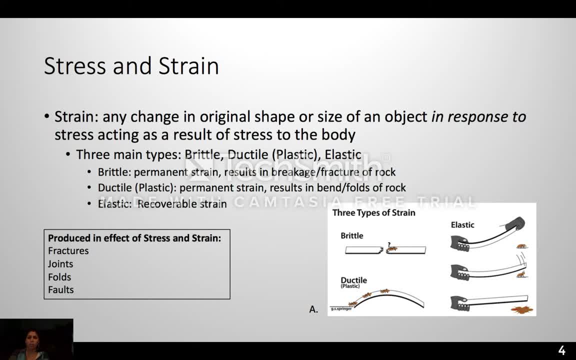 However, with this strain, while the stress still exceeds the strength of the original strain, the rock will not break. It will just fold or bend. Lastly, the elastic strain is a recoverable strain. While it may stretch, it is capable of recovery to its original form. 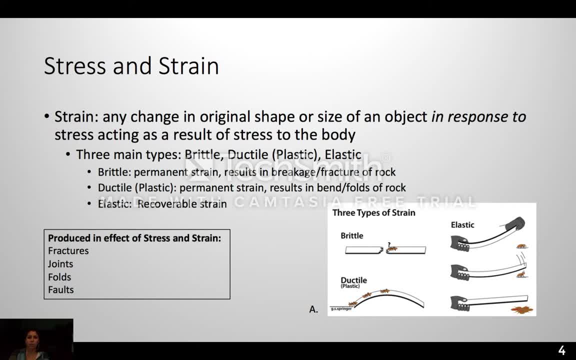 It is not permanent. After the effects of strain, stress and other environmental factors that affect deformation that I mentioned before, we can begin to name a few of the geologic structure's deformations. Let's start out with fractures, joints, Folds and faults, to name a few. 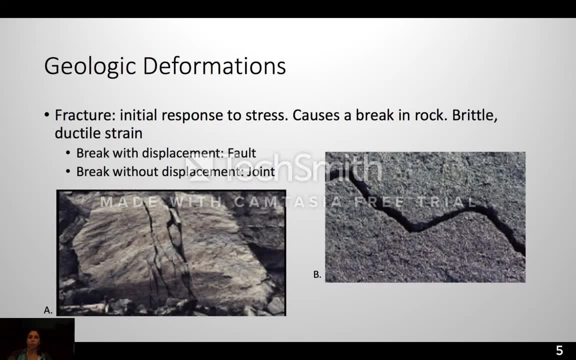 Fracture is the initial response to any type of stress or strain. Such fractures can be described by observing if there is displacement, which means that there would be a fault, or no displacement, which would suggest a joint had occurred. Both of these pictures, as you can see, are of fractures with very little to no displacement. 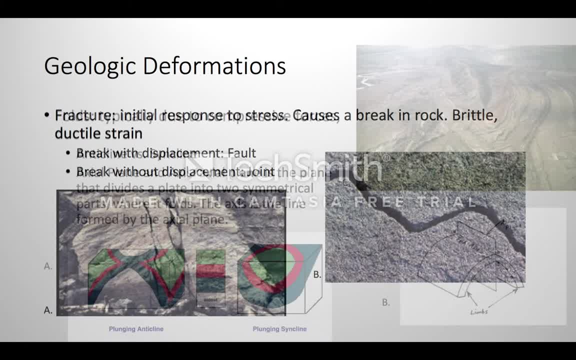 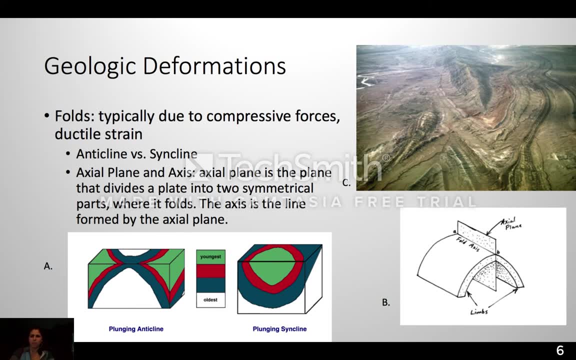 So we can just assume that these are joints. Folds are typically deformations. They are due to compressive forces. Looking specifically into folds, some terms to recognize are: endocline vs incline, axial plane vs axis, horizontal vs plunging. 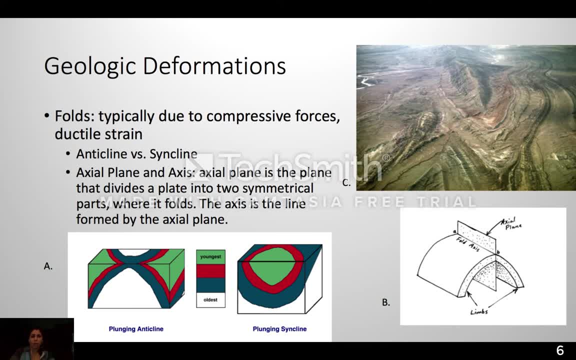 and dome vs basin To start off. an endocline fold happens when the older rocks fold on the inside. A syncline fold occurs when the older rocks fold on the outside. As you can see in the image, the endocline is on the left. 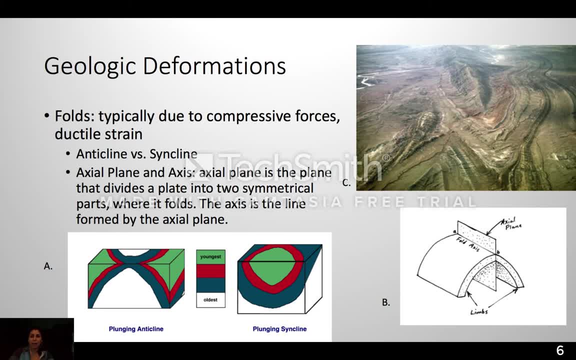 where the oldest, or white rock is on the inside and the syncline, where the older rock is on the outside is on the right. More specifically, about folds. the axial plane is the plane, that which divides a plate or piece of rock into two symmetrical parts. 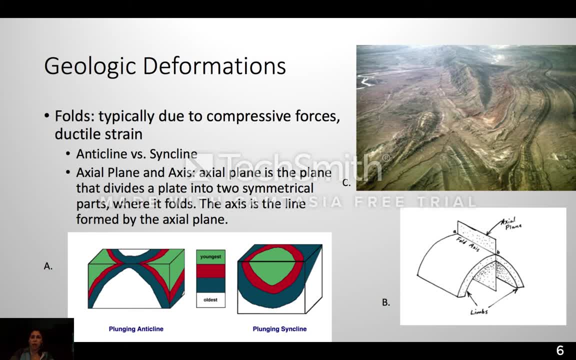 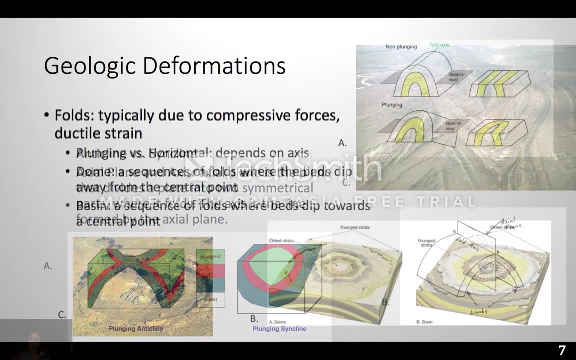 where it folds. The axis is the line formed by the axial plane, as you can see in the picture, Figure B. Figure C is in a picture of an area in Wyoming where there is a beautiful plunging endocline. As we learn more about folds- a horizontal or a non-plunging fold- 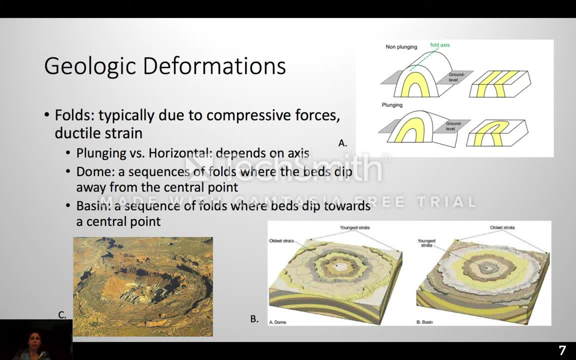 can be described as horizontally folding and the axis being horizontal, while a plunging fold's axis is not horizontal. It is either vertical or diagonal. You can typically see the plunging arcs in the earth, like in the picture on the previous slide in Wyoming. 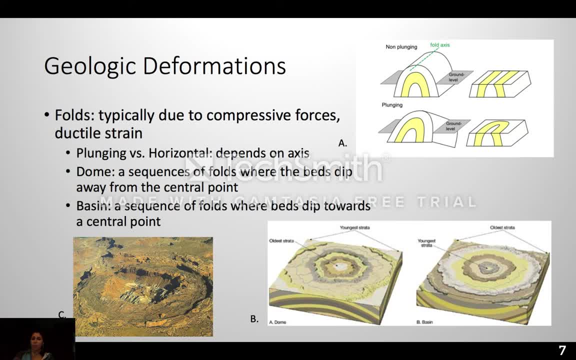 See how it matches up with Figure A. the picture from Wyoming looks identical to the plunging formations in Figure A. That shows that is a beautiful example of a plunging fold. Folds can also create formations like domes and basins. A dome is a sequence of folded rocks. 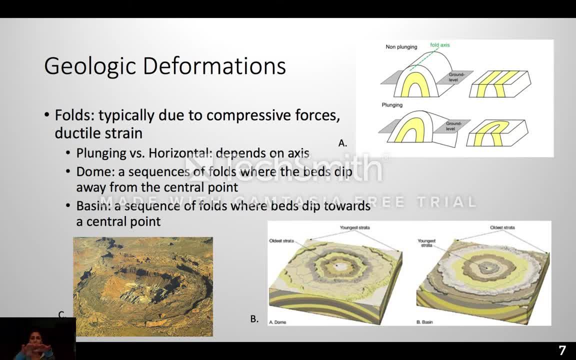 where the beds dip away from the center point like an overturned bowl. Older rocks are in the center and younger are on the outsides. A basin is the opposite, where there is a sequence of folded rock beds who dip towards the central point like a normal bowl facing up. 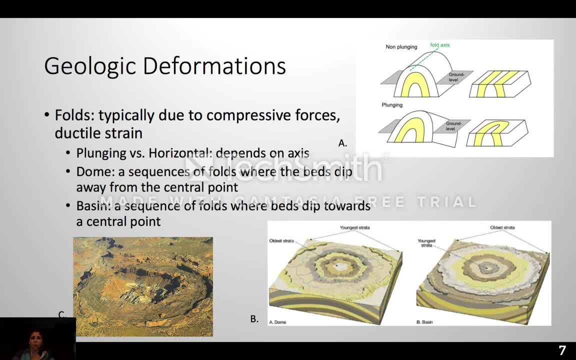 Here the youngest rocks are in the center, while the older are on the outside. The Year C is an example in a picture of the upheaval dome in the Canyonlands National Park. It actually used to be able to see the dome more clearly. 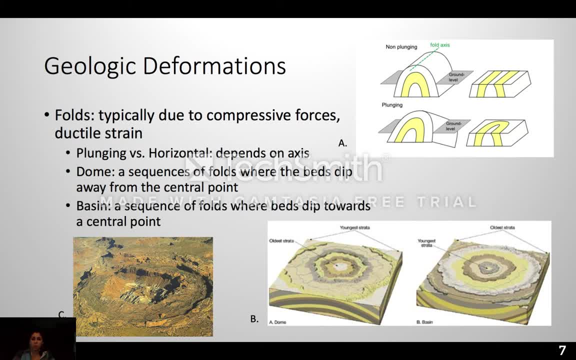 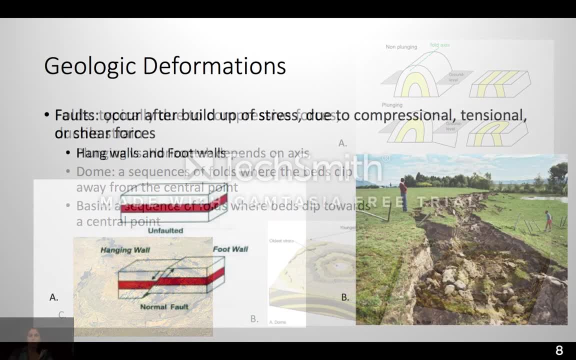 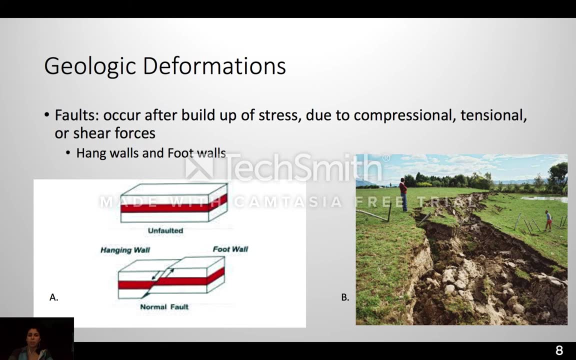 but the central area has eroded, but you can still tell it is a dome because the oldest rocks are found in the center. Folds typically can occur after a significant amount of stress builds up in the crust. They can be due to tension, compression or even shear forces. 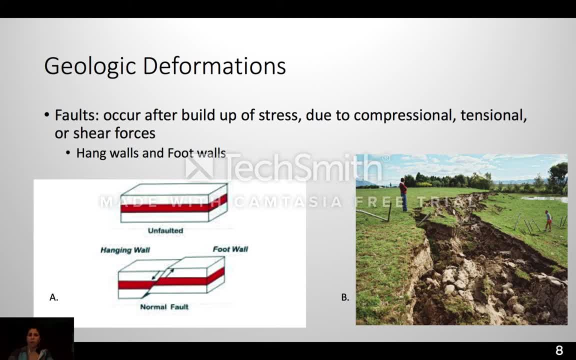 all of the different types of stress. A fold can be created and a rock can shift several meters in a second. This can be most easily identified as an earthquake, as we see on the news and all around us every day When folds split the crust. 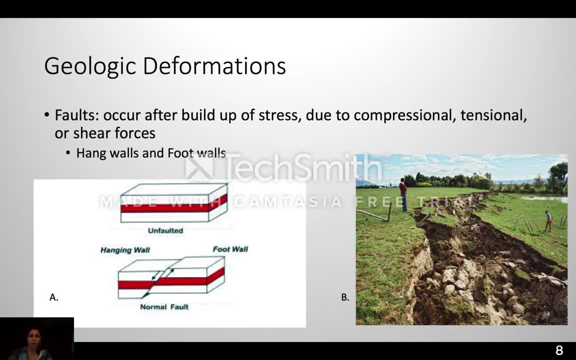 they create hang walls or foot walls. This is a way to describe how the crust split diagonally. For example, if the base of the rock structure comes out further than the top, then the fault can be classified as a foot wall geologic structure. 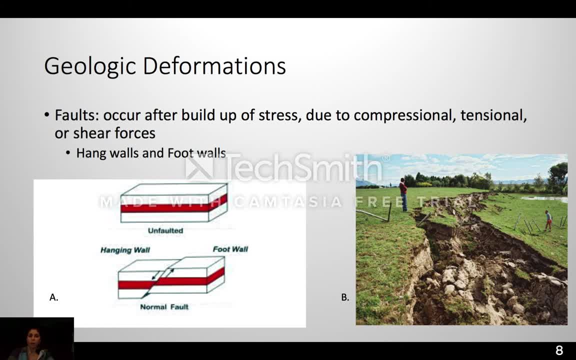 However, if the top comes out further than the bottom, then the fault can be classified as a hang wall geologic structure. As you can see in Figure A of a normal fault, the hanging wall is on the left and the foot wall is on the right. 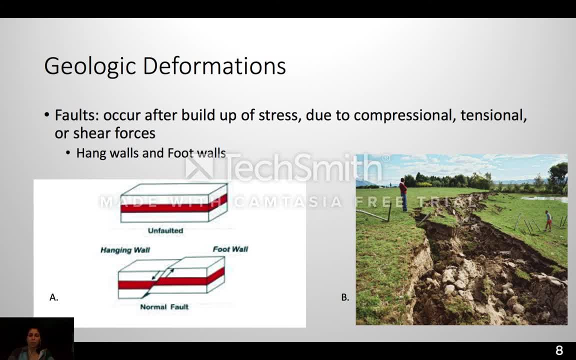 The next picture in Figure B is a picture of an earthquake in Edgecombe, New Zealand, in 1987. Here a fault ruptured the surface and the northwest land to the fault sank 2 meters, as you can see, as it is below in the picture. 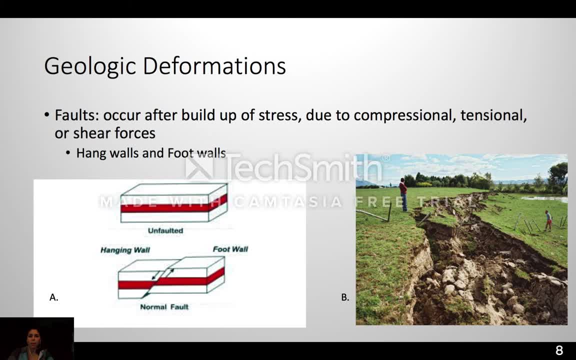 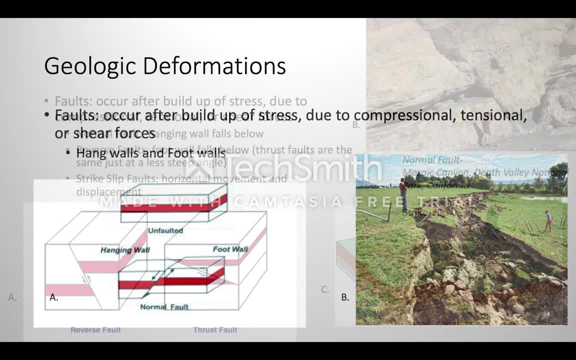 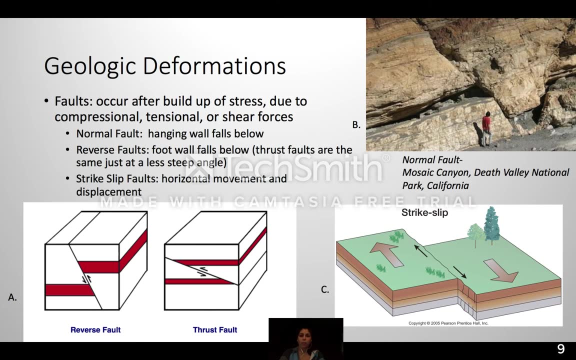 We can learn how to classify this event by further analyzing how this fault moved and which parts- either the hang wall or the foot wall- moved up or down. And now we turn to ways to describe faults. by how they move, A normal fault is when the hanging wall has fallen below the foot wall block. 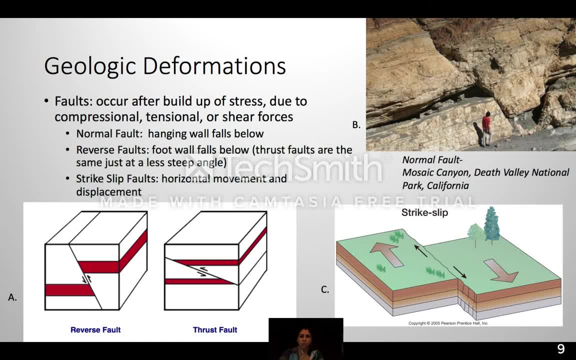 This normally can occur due to any type of tensional stress. A reverse fault is when the foot wall falls below the hanging wall, And here dip angles must be greater than 30 degrees from the horizontal, so it should be a pretty steep one. 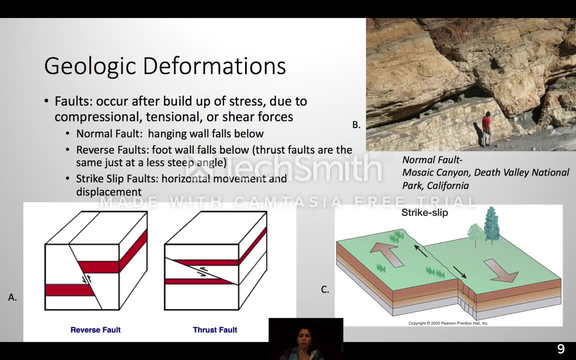 Thrust faults are basically the reverse, just with dip angles less than 30 degrees from the horizontal. so this is a less steep type of reverse fault. This is typically due to compressional stress. Lastly, the last type of fault is the strike-slip fault.